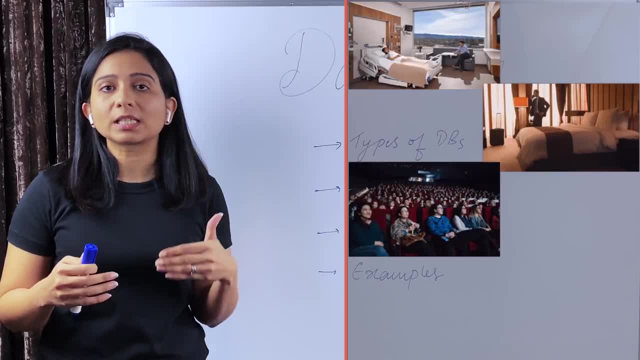 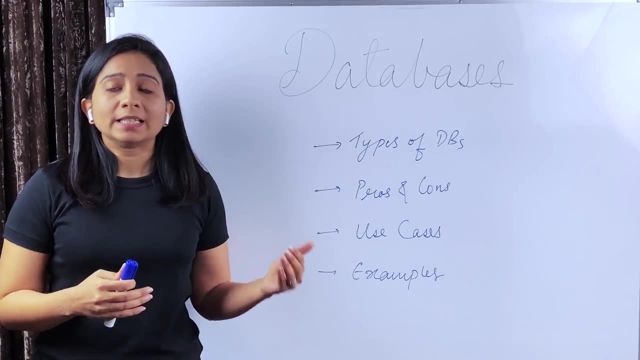 theater, there are chairs lined up in front of the screen so that people can sit and watch a movie. In malls, there are big, large spaces so that people can move around. Similarly, different databases depending on the property of data and the volume of data querying requirements. 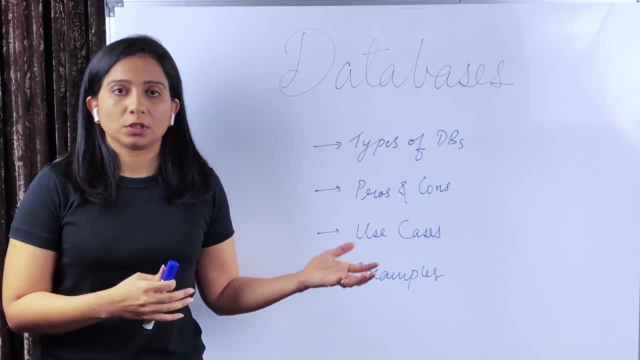 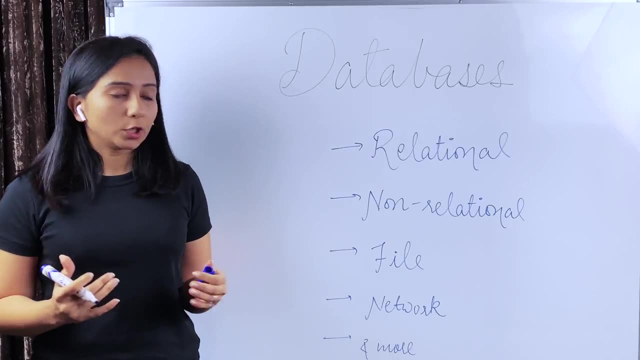 provide different features and the way to store data. So in this video we are going to see how those different types of database provide and fulfill such requirements. Some popular type of databases are relational, non-relational file type, dbs, network dbs, etc. In this video we are 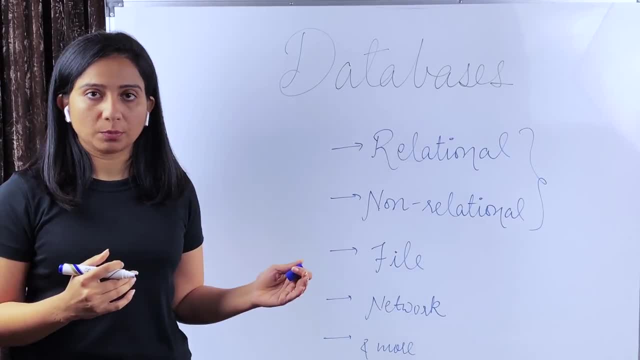 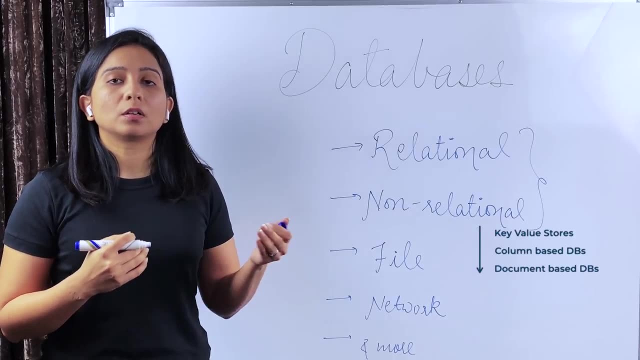 going to focus on relational and non-relational dbs. Non-relational dbs are again divided into multiple types like key value stores, column based dbs, document based dbs, search dbs, etc. So we will look into those examples as well. Relational dbs are the most popular ones. 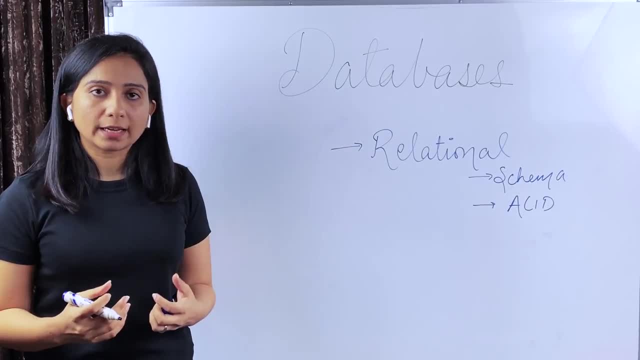 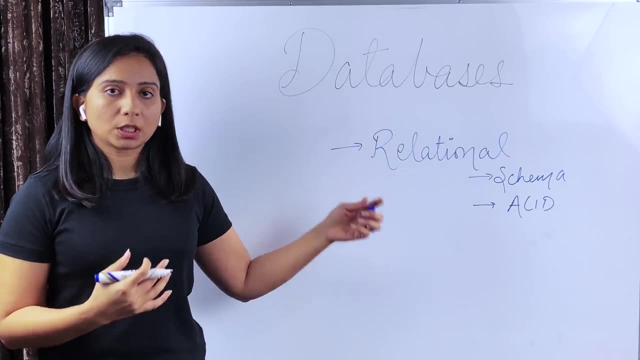 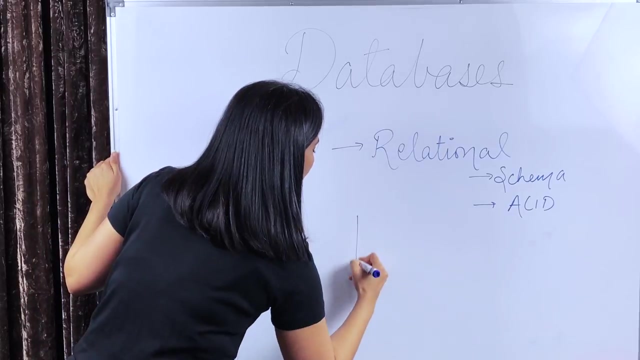 and here are the two factors that help you decide whether you have to select a relational db for your use case or not: Schema and asset properties. Let's talk about schema. Schema in relational dbs refers to how your data is going to be structured. So in relational dbs you have 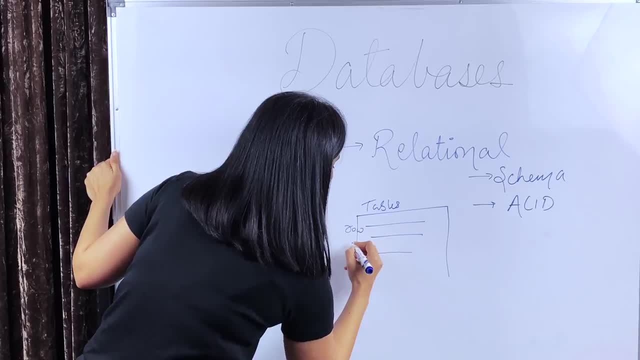 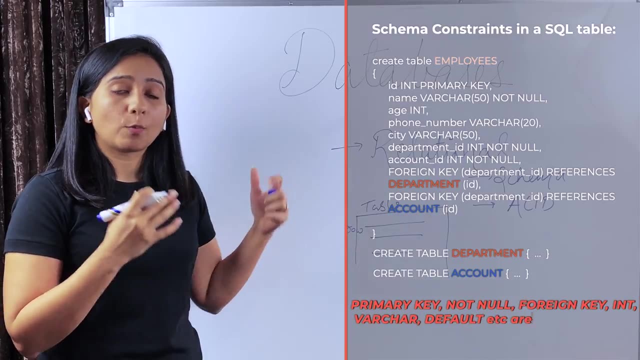 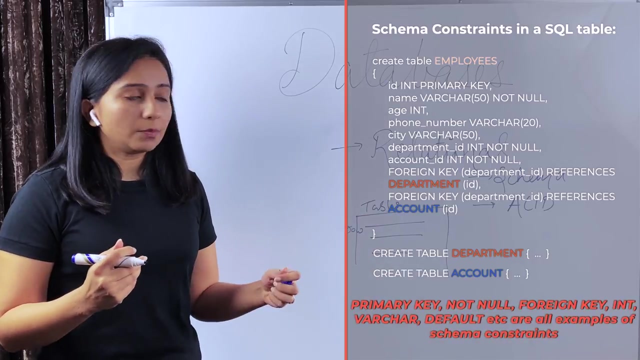 tables and rows which store the data. So if your data can be represented in the form of tables and rows while satisfying the property of relational dbs- like if your data is complex and it could be represented using relational tables easily- then you select relational dbs. A classic example is: 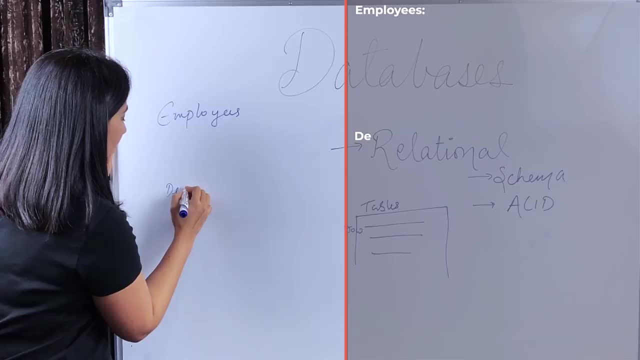 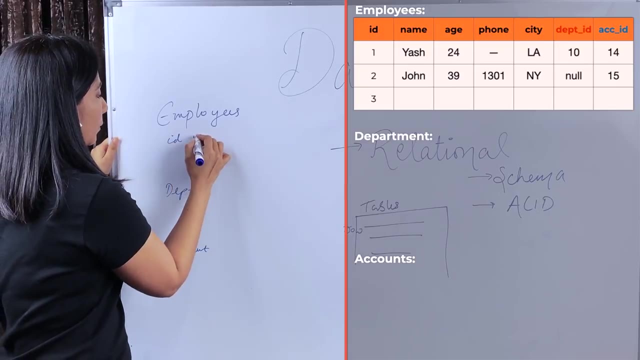 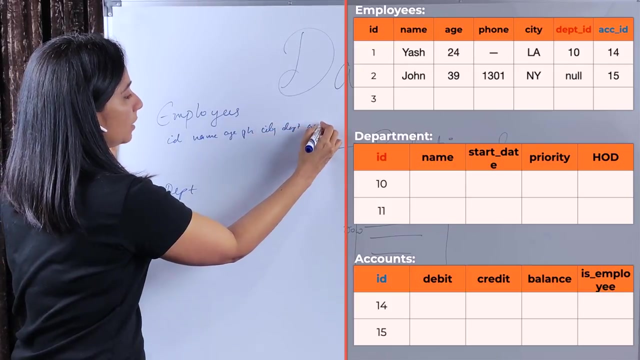 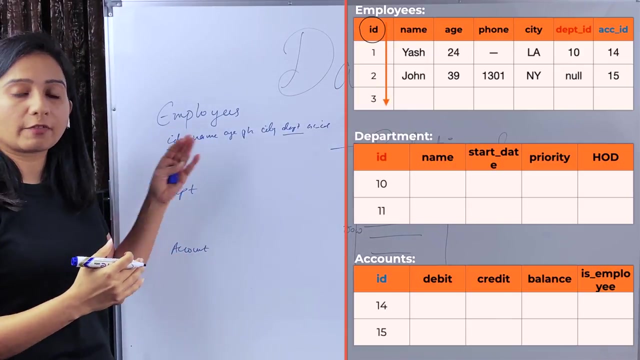 employees data. So you have an employees table, a department table, an account table. So employees data is going to store the data of employees, like name, age, phone number, city, department ID, account ID, etc. Now this ID refers to the primary key or the unique ID which identifies every. 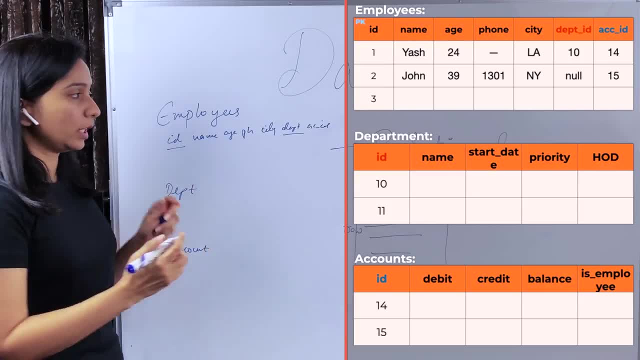 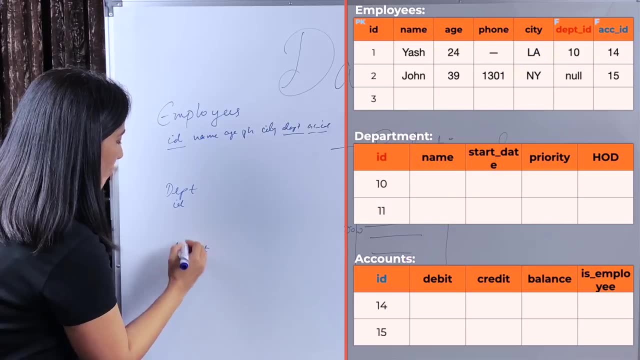 employee and department ID and account ID are foreign keys, which identifies which department this employee belongs to and what is the account ID of this employee. So these are called foreign keys. So the department table will have details like the name of the department when it was. 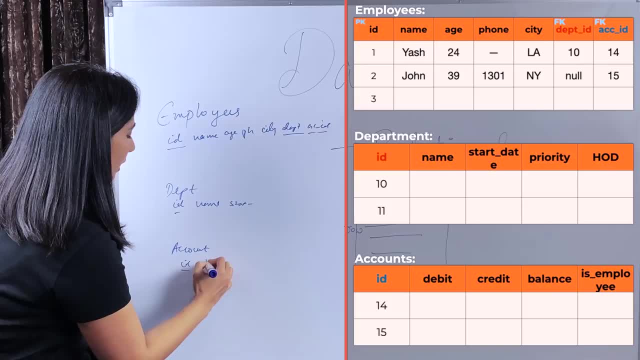 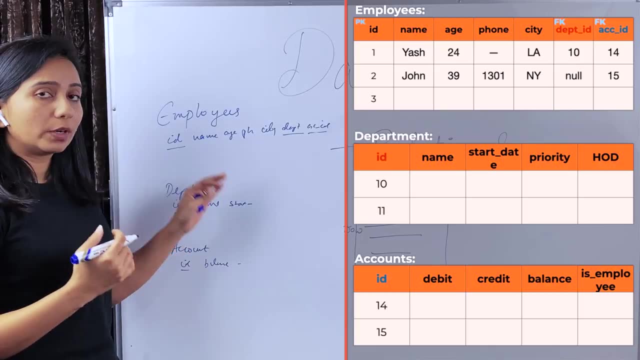 started and other details. and account ID will have other details like balance and so on. Now how schema constraints come into the picture. Employee data will have requirement that one employee has to belong to a department and that employee has to have an account as well. So department and account. 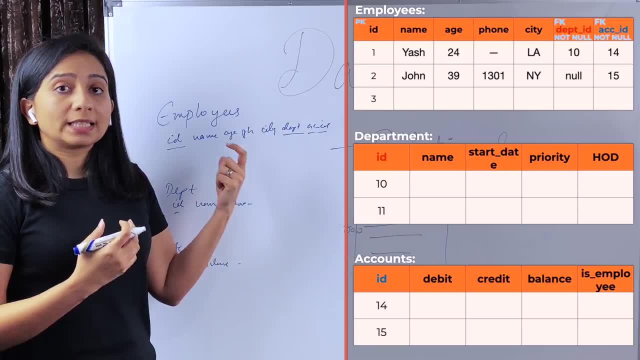 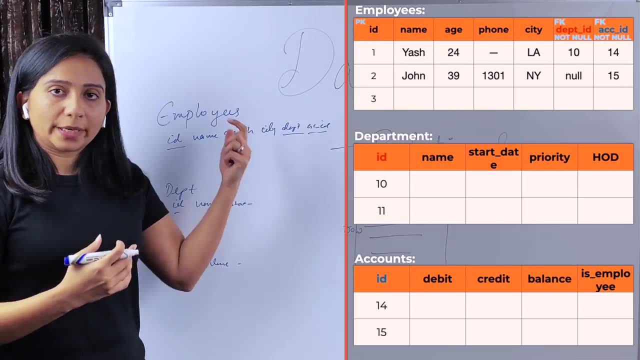 cannot be null. That is a schema constraint and if your data can satisfy that- and you know that, that this is going to be the structure of your data- we make the decision of selecting relational DBs. What are the benefits of this? relational DBs or schema One you can represent? 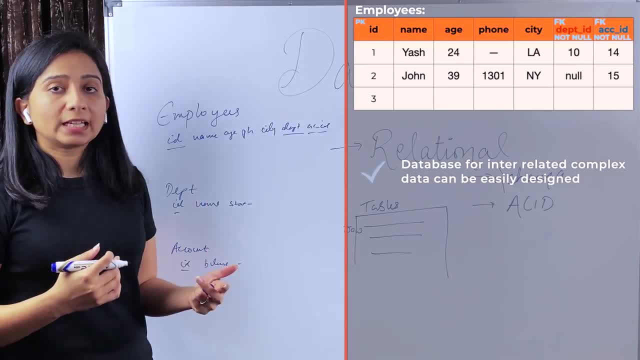 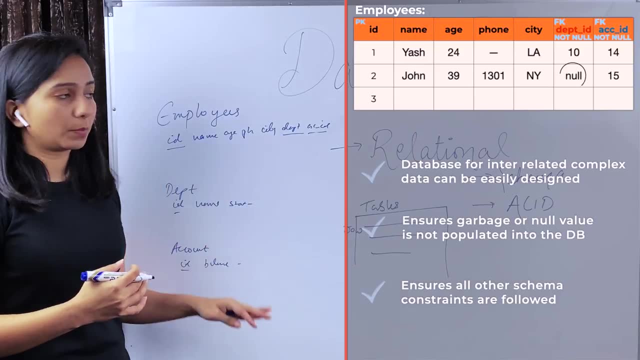 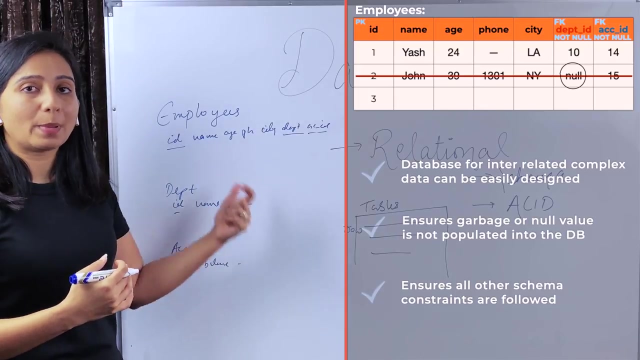 complex data easily using relational tables. Second, with the schema constraints, you can ensure that some garbage data or null data doesn't get into your database, because the schema constraint- like department ID cannot be null, account ID cannot be null- will ensure that you don't have inconsistent data or bad data in your database. Talking about asset properties, if you 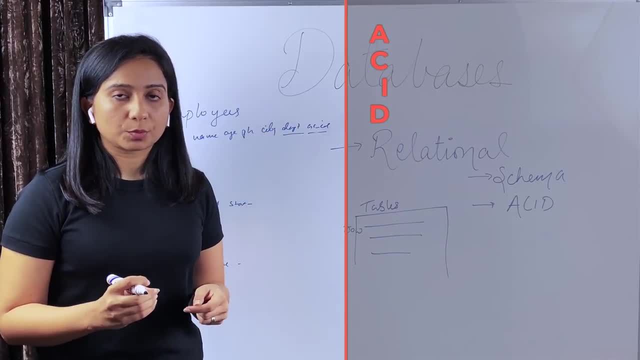 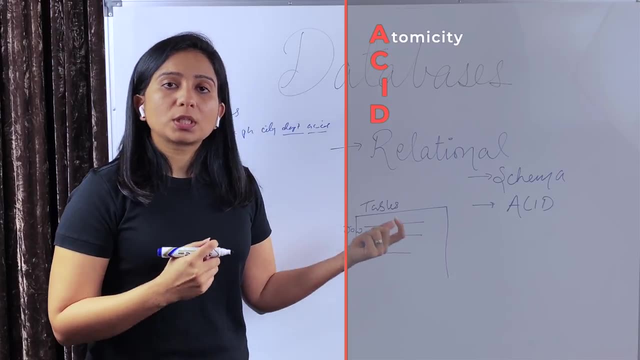 don't know what are asset properties. I have included a link in the description box below, So in the description, but still i'll cover basics of asset properties. so a in asset properties stands for atomicity. atomicity means a transaction in a database either happens completely or doesn't. 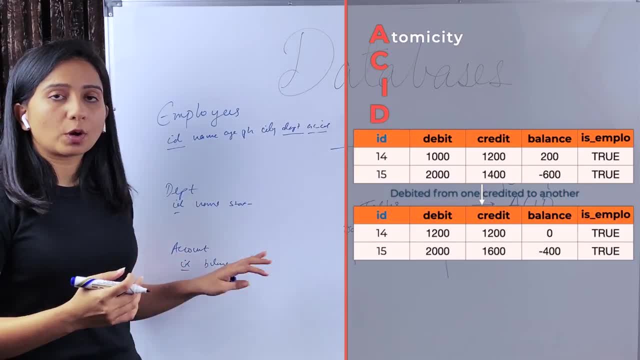 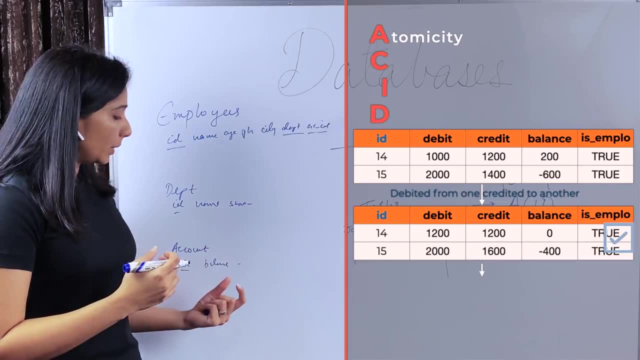 happen at all. so, for example, if you have to transfer money from one account to another account, the transaction should deduct money from one account and put money into the another account. but it should not happen that it deducted from one account and didn't update into the another account. 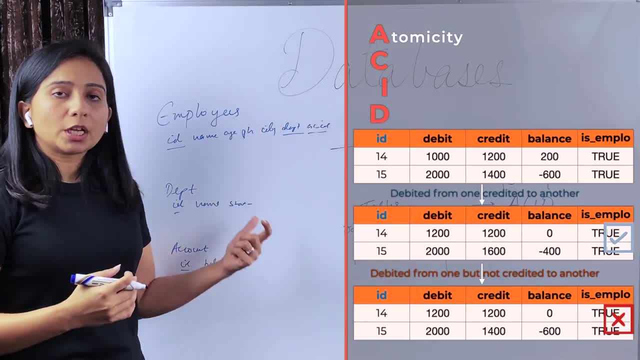 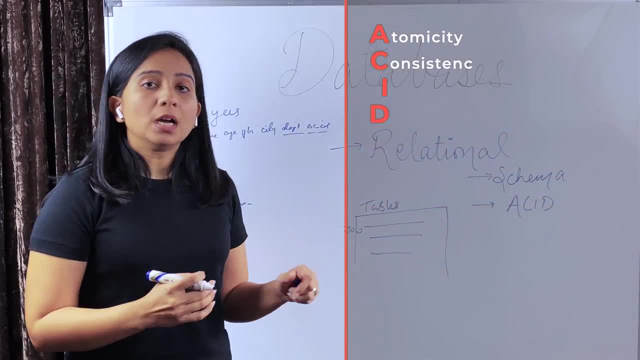 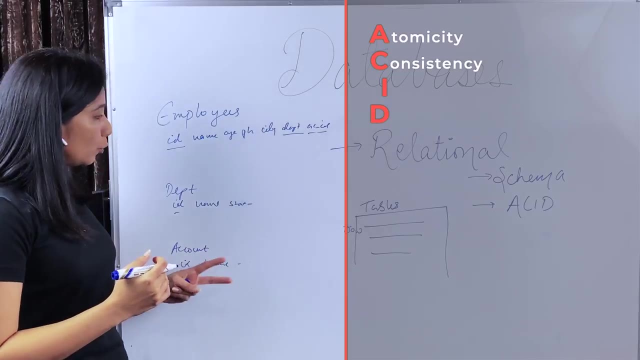 so that is breaking the rule of atomicity. relational dbs ensure that all the transactions are atomic. either they happen completely or they don't happen at all. second is consistency. consistency means that at any given point of time the state of the database will be consistent. it will not happen that if two reads are happening, if two requests are trying to read the account, 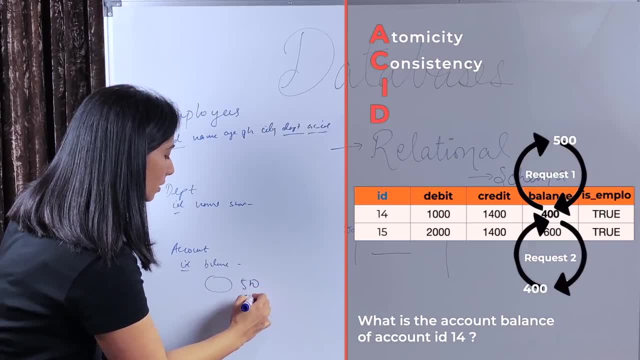 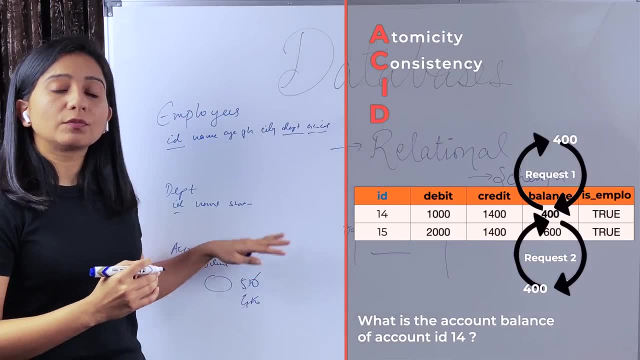 balance. one request gets the response as 500 and another gets the response as 400. this is not possible if the db supports asset properties, because your database is not consistent with the state of the database. so that is breaking the rule. of atomicity is consistent, it will give the same value to both the requests then. 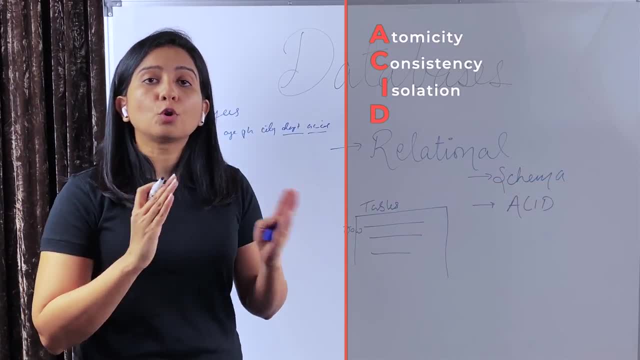 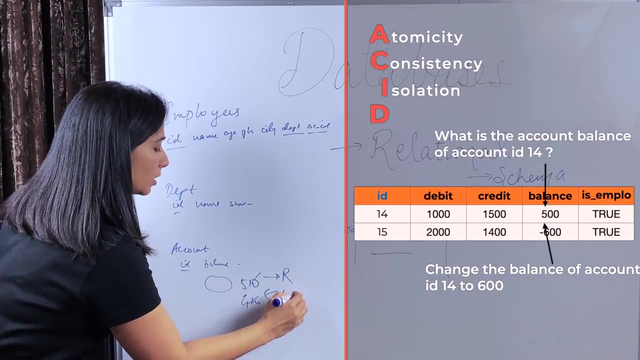 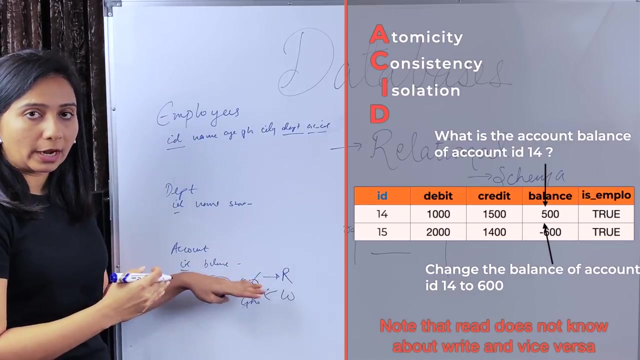 isolation. isolation means the two transactions do not know about each other. for example, there is a read happening on the balance and at the same time there is a write is also happening. suppose when read is happening, read will read the older value, like 500, until the write is completed and write will go and 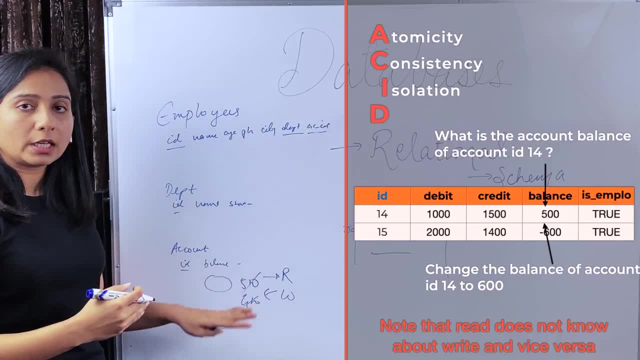 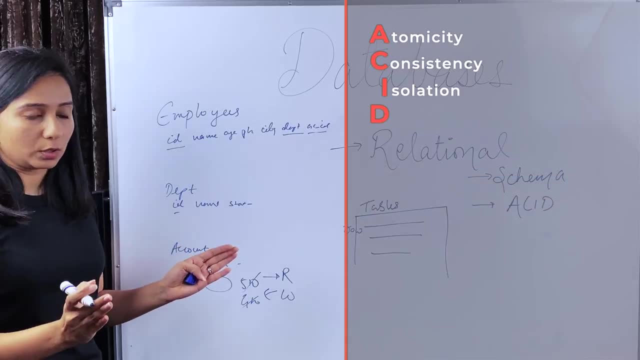 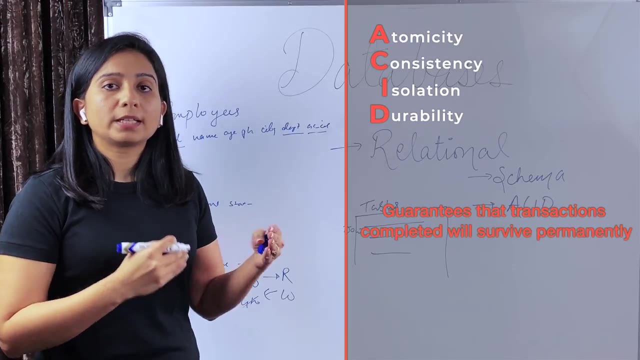 update that value to 600. if the read happens after write, it will get 600. if the read happens before write, it will get 500. read would not know about the write operation. so this is called isolation, then durability. durability is a mechanism that database ensures whatever writes or updates are happening. 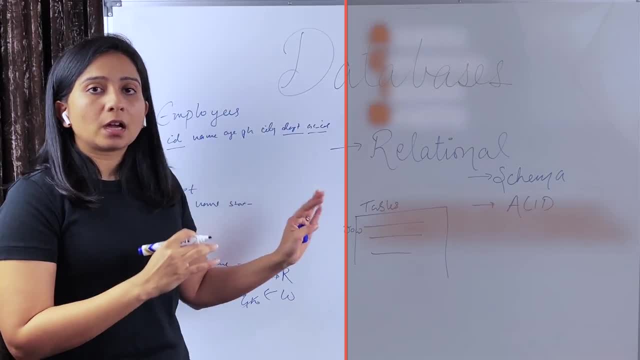 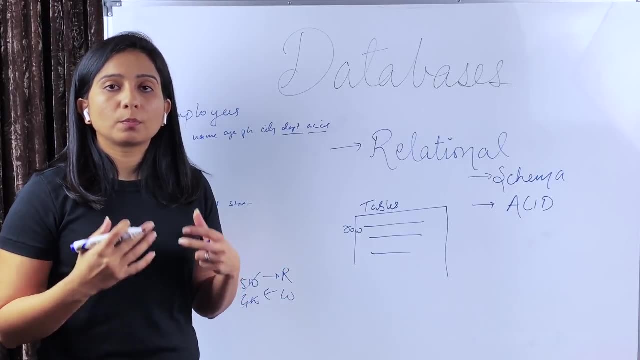 they are logged properly and all the details and the data is getting persisted into the disk storage. so that is just a brief of asset properties. now, if you have to support your business requirements as per asset properties, if you have the need for transactions or if you are building like a 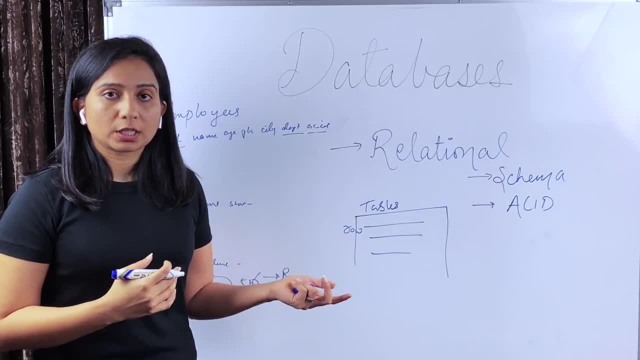 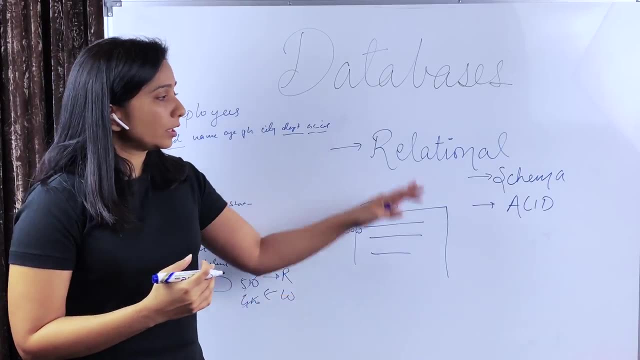 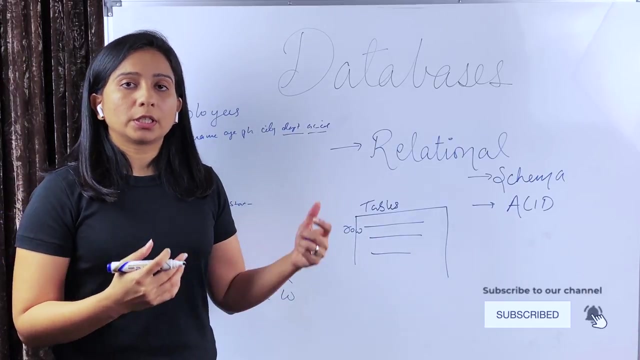 banking application which has a requirement for transactions. then, and also if you have a fixed schema which is not going to change in future, as much, you select relational dbs. what are the things that relational dbs cannot support? for example, you have a certain kind of data in which 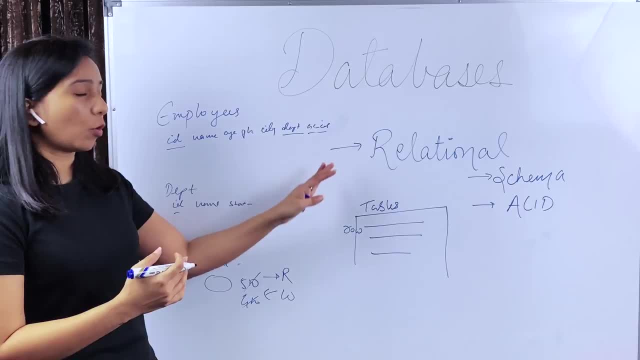 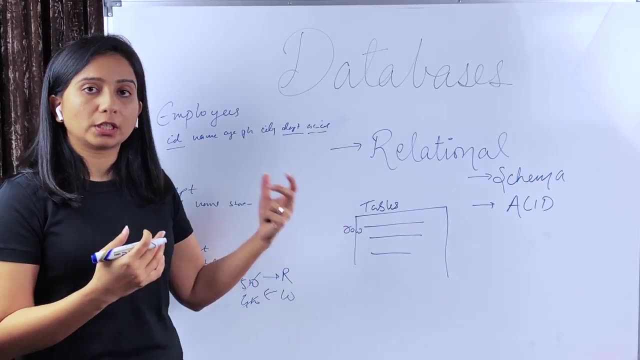 this schema is not fixed. you do not know what are the different columns or fields that could evolve as your product evolves and you're not sure that how your, how the schema of your data, is going to evolve. in that case, using relational dbs becomes a little difficult, although there are. 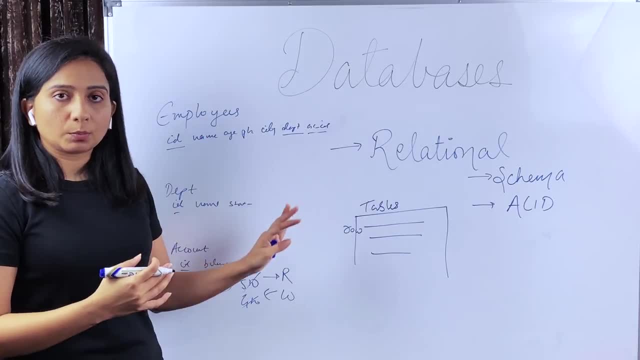 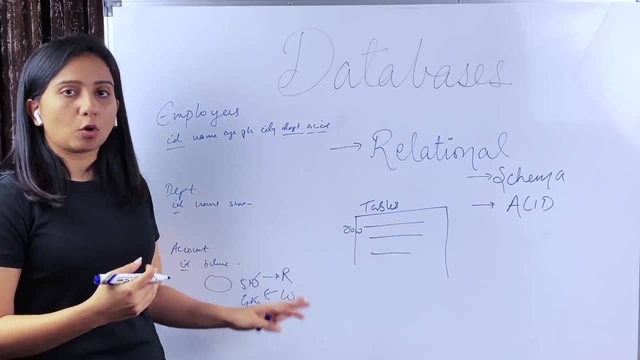 ways to update columns and change the schema of the table. but if, when the table size grows and the data set becomes huge, it becomes increasingly complex to add new columns, and also when the data size grows and the queries require multiple properties to be fetched from different tables, 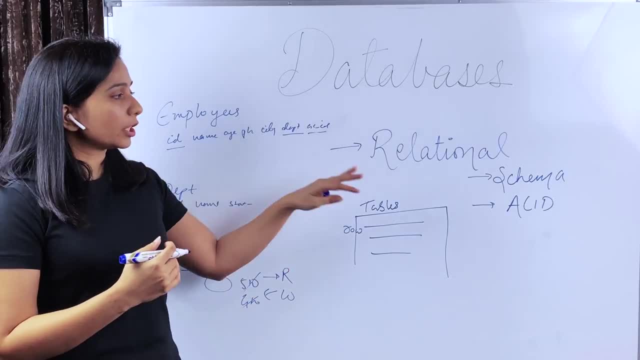 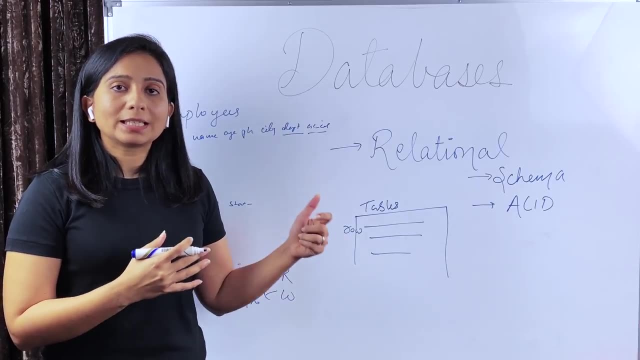 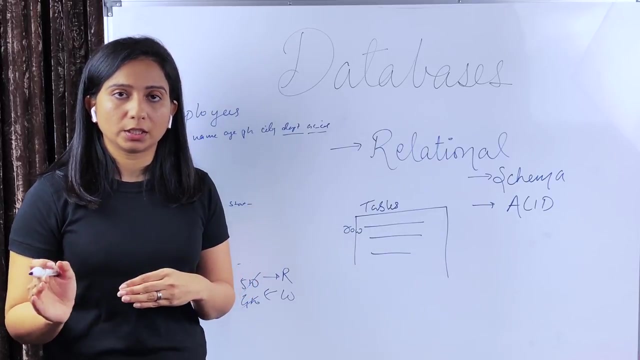 the joins can become expensive. so that is the case when relational dbs don't show much performance as expected. second part is scaling. in case of relational dbs, it is easy to store or scale vertically. we are going to discuss vertical scaling or horizontal scaling in detail, but right now just understand vertical. 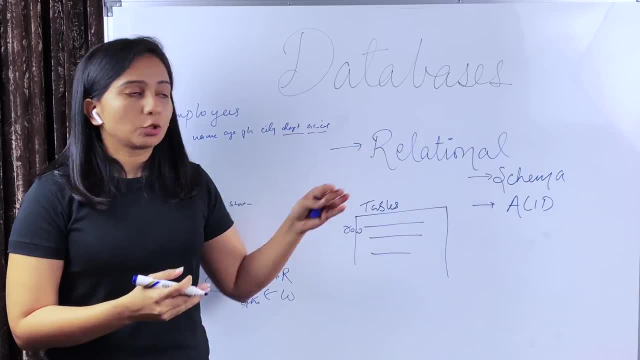 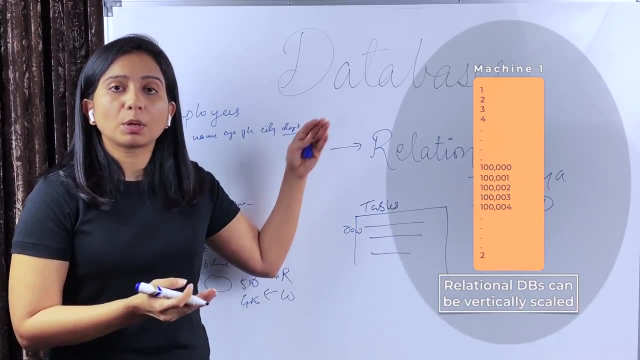 scaling means you can increase the storage of one machine. so suppose if you have a table that has, say, 1 million rows, when you foresee that it is going to grow to 2 million rows, you can increase the storage of one machine. but in case of relational dbs it becomes difficult to divide that table and 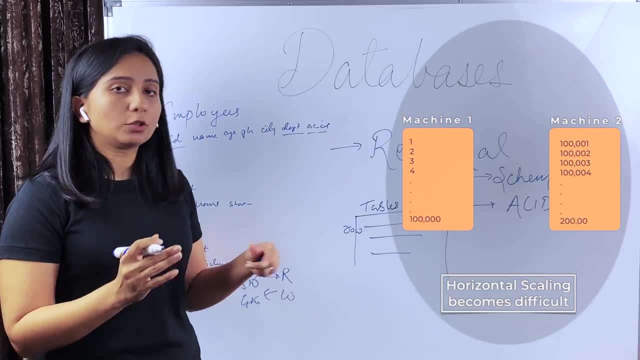 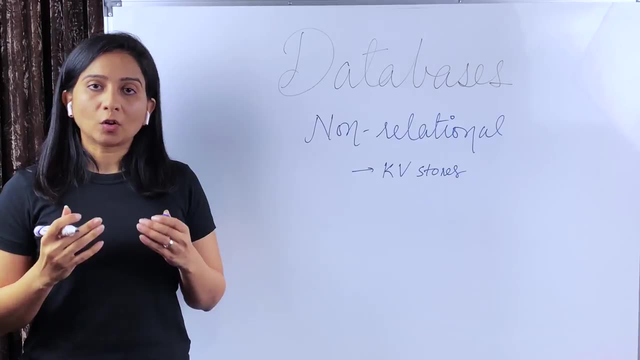 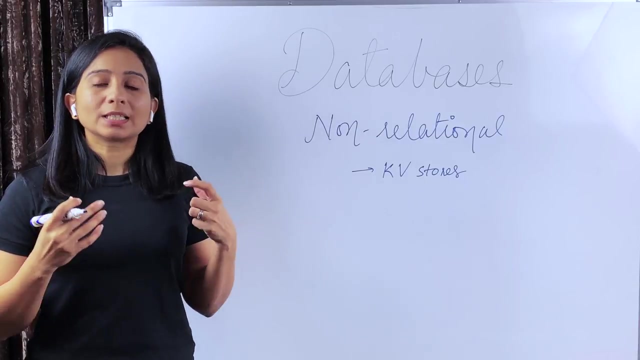 put it on two different machines. there are ways to divide the table through application code, but it is difficult to perform horizontal scaling in case of relational dbs. now let's talk about non-relational dbs, or sometimes known as no sql dbs. in such databases, the schema is not fixed and different. 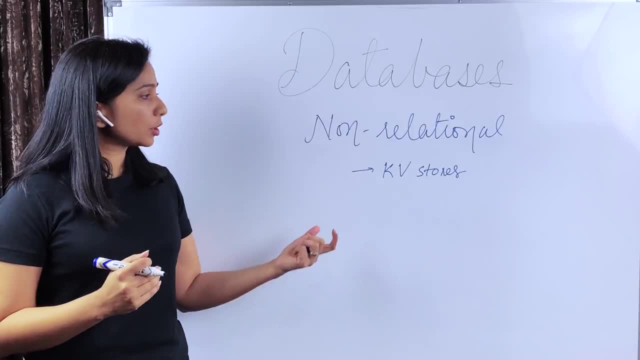 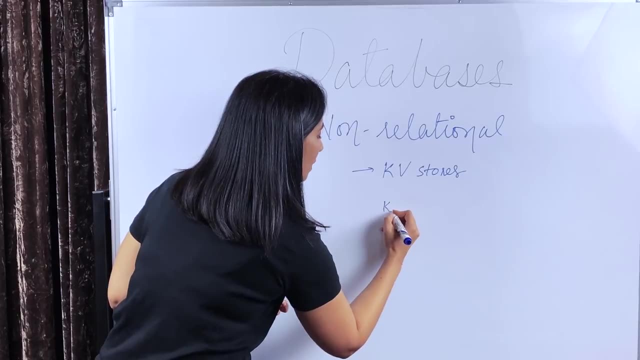 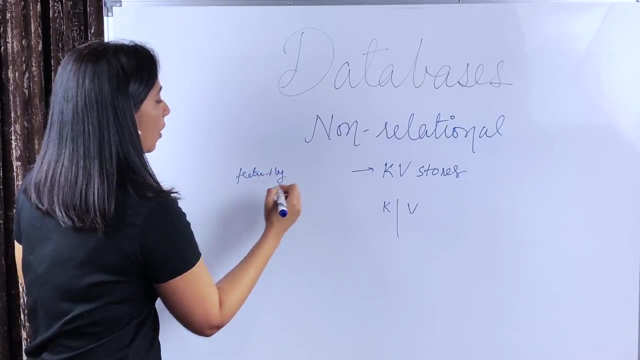 types of non-relational dbs cater to different requirements. let's first talk about key value stores. key value stores have just, uh, like a hash map. it will just have a key and a value. so suppose you have requirements, like you have a feature flag or you have certain. 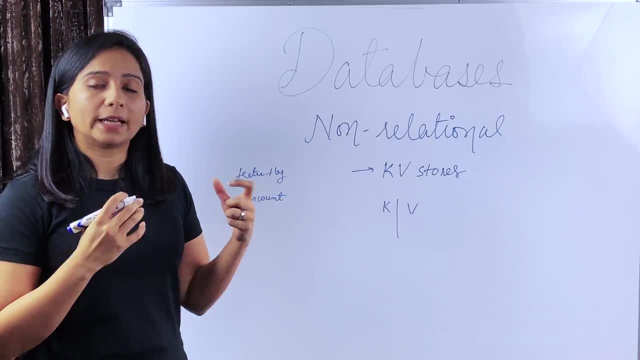 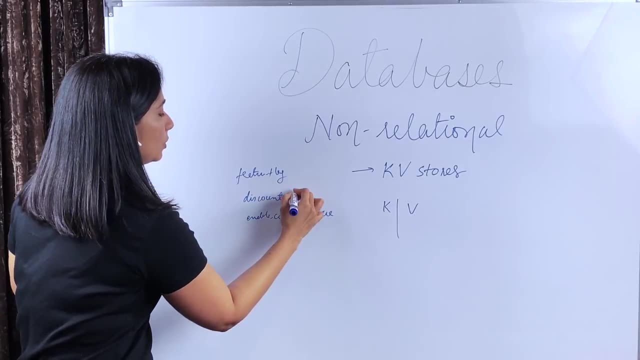 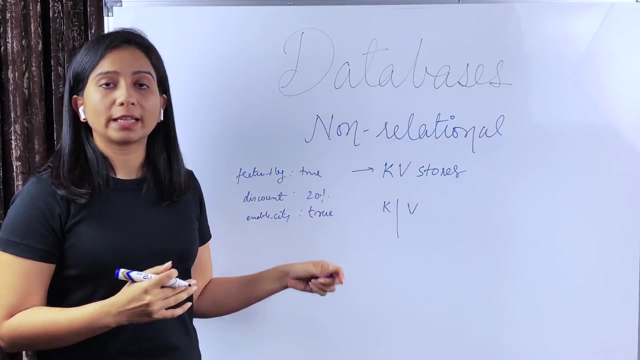 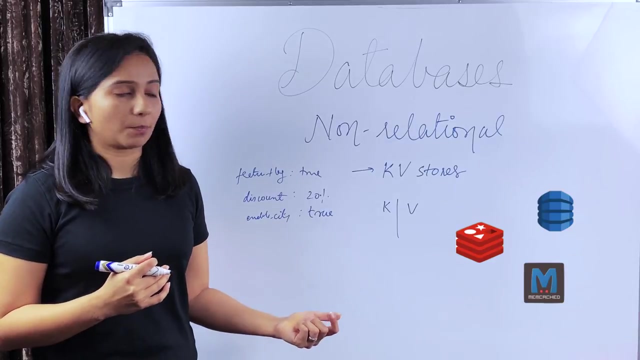 discount or promotion, or you want to enable certain feature in a certain city for your application, so these kind of values could be stored in key value stores. there are multiple other cases for key value stores, like caching. solutions are implemented using key value stores. some examples are redis, dynamo, db, memcache, etc. the benefit of key value stores is they are quite fast and they 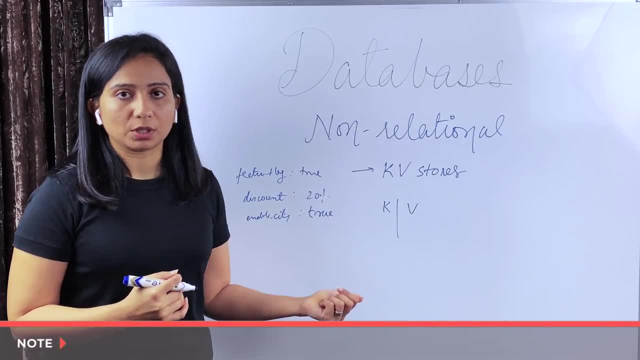 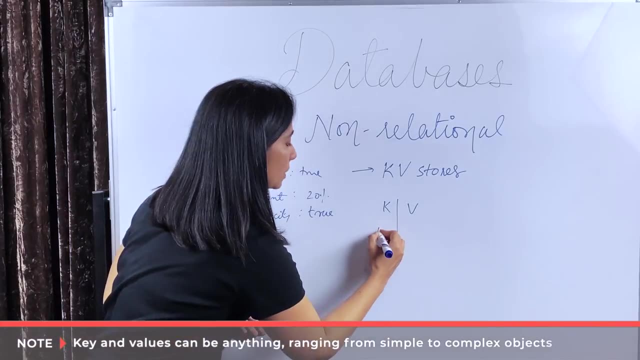 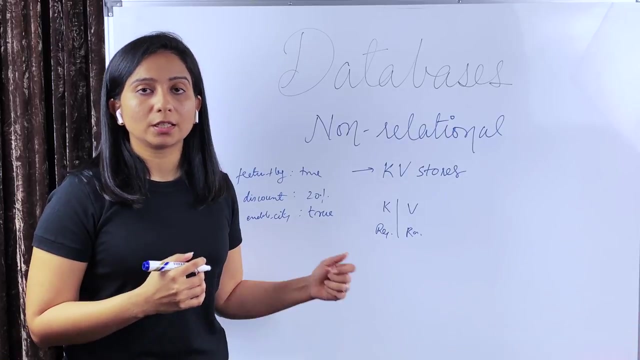 provide quick access because most of the data stores are in memory. apart from such kind of data like application related data or configuration related data, you can also store, like request response, into key value stores. again, key value stores could be used in multiple caching solutions, which we will discuss in detail in the caching video next. 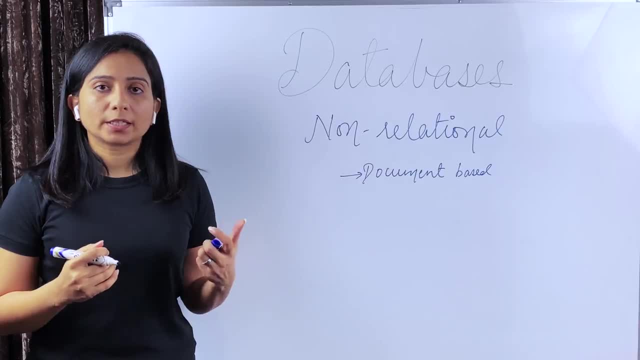 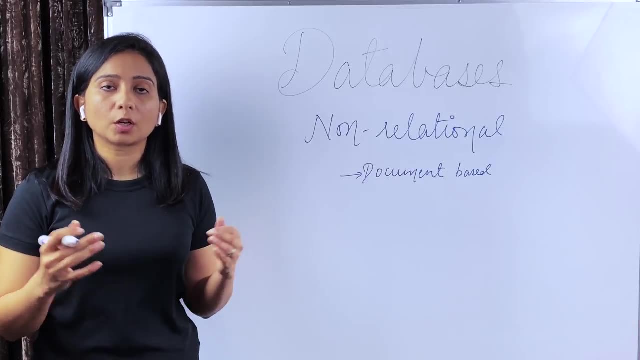 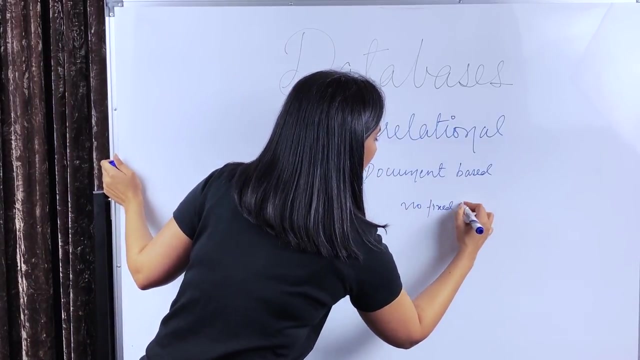 let's talk about document based databases. document based databases are usually used when you are not sure of the schema or how the data and the fields- different fields of data- are going to evolve over time. in such cases, document based dbs are used. so there is no fixed schema. and one more important: 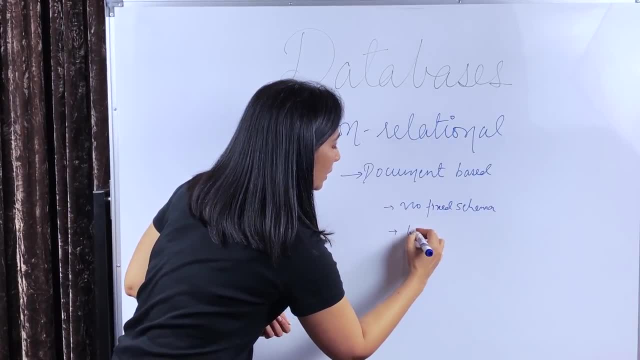 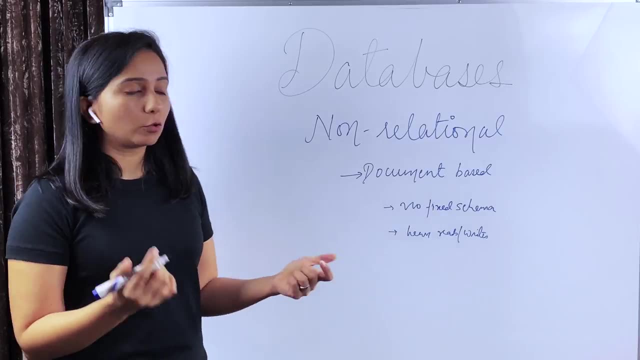 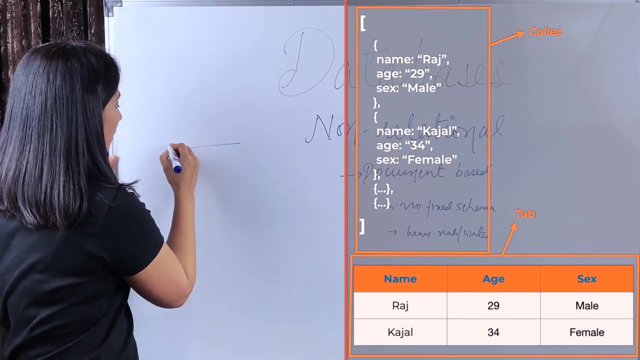 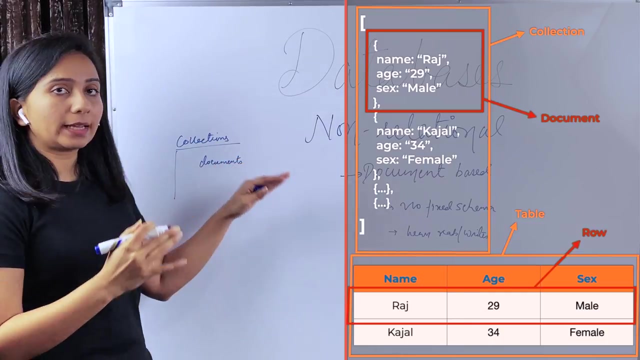 point for document dbs are they can support heavy reads and writes. so let's see how a document based db looks like. just like in relational dbs, we have tables and rows. document dbs have collections and documents, so you can think of documents as rows and collections like tables. the use cases. 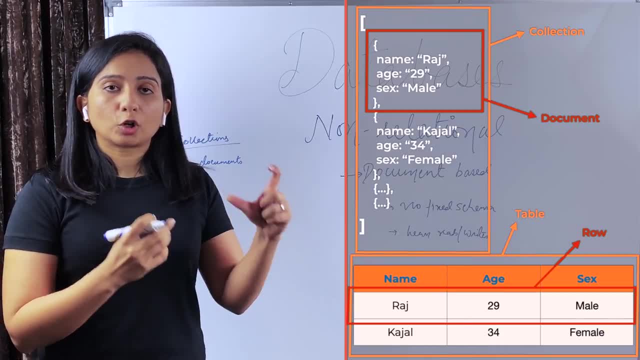 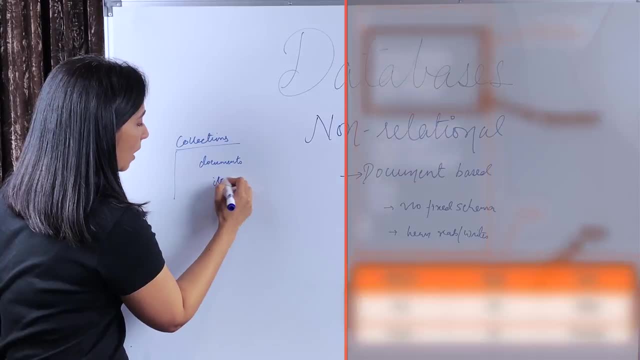 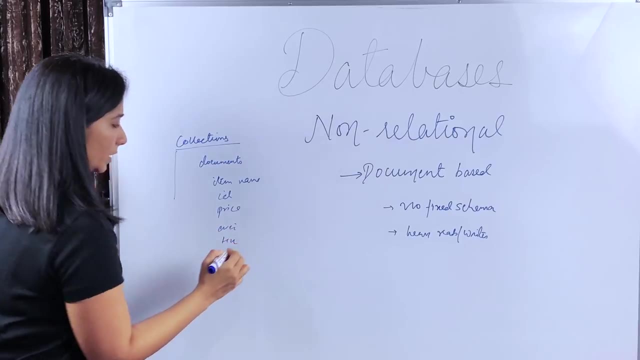 like when you have to, for example, store a product details, like for an e-commerce website. if you have to store product details for an item, so you will have item name, item id, price, availability, tax, etc. some, some details like that. and you know that these details, although are 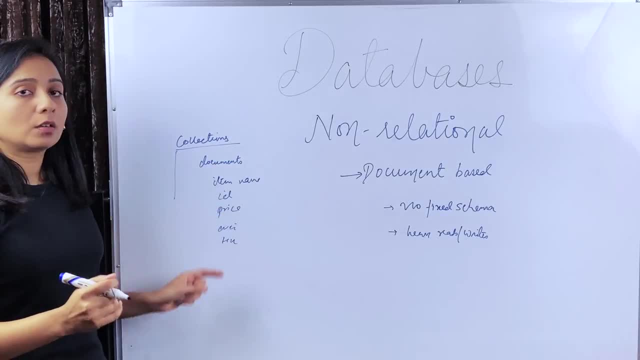 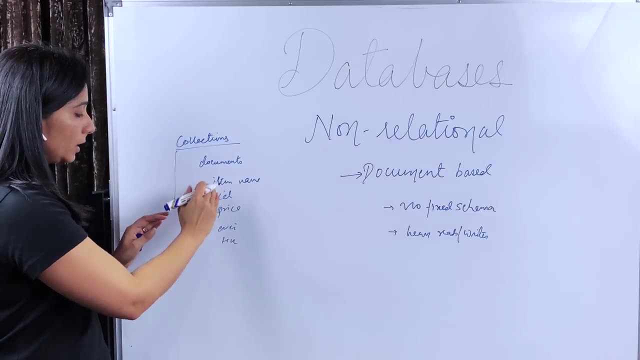 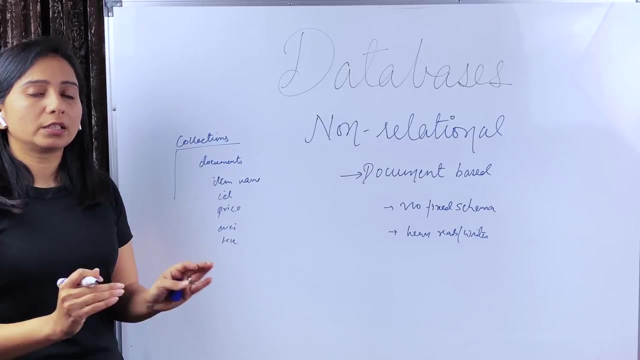 known, but they can change over time. also when querying such kind of data you would need all these properties at once in one query, so you don't want to have this different data in different tables and then make joins and fetch the data. so document dbs help you in decreasing that complexity. 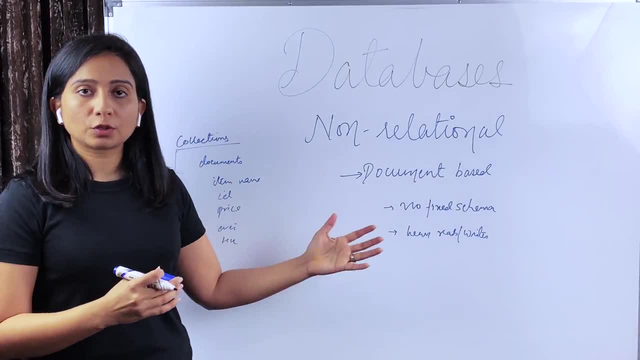 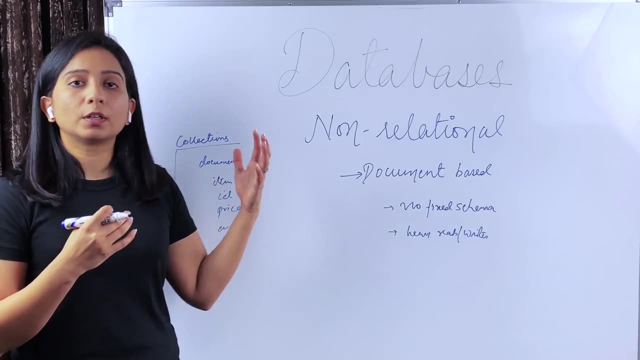 so when you have use cases like that, the schema is not fixed. you don't know how it is going to evolve over time. you want that flexibility of keeping dynamic data and also when you have the use cases for heavy reads and writes. in such cases, document dbs are a choice. let's take one more. 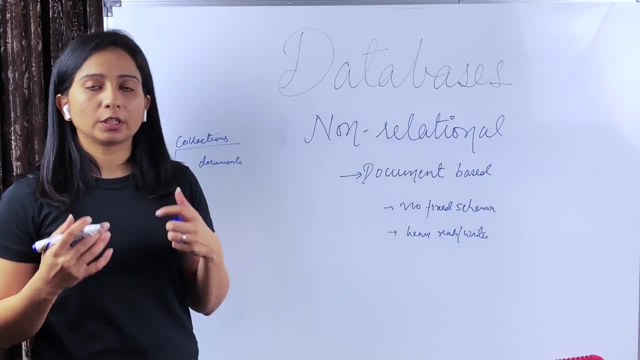 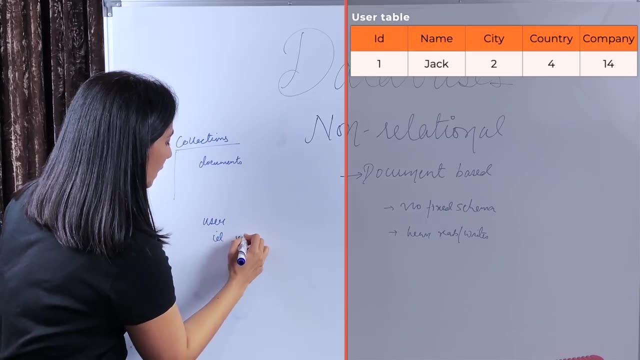 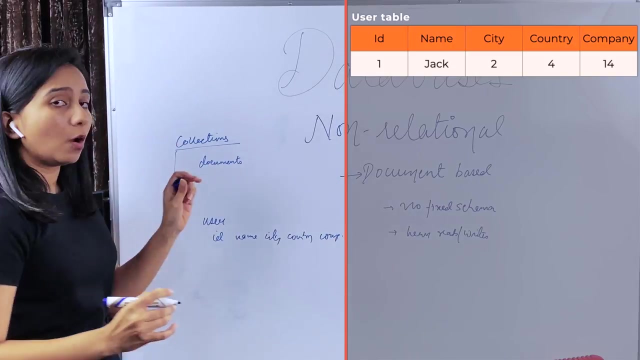 example to make it more clear. suppose you have a relational db where you store user related data. so you would have a user table where you have user id, name, city, country, the company he works for, etc. if you have to fetch all the user details, you would have to make query. 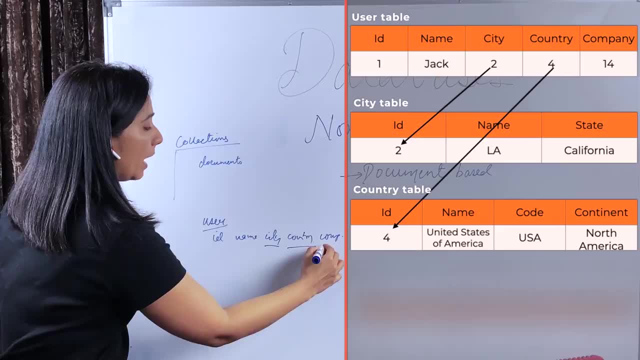 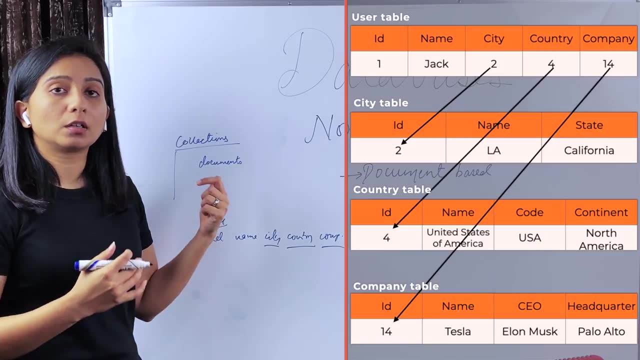 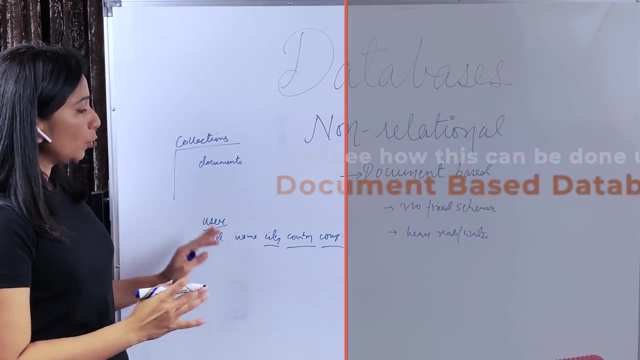 to user table, then city table, country table and company table to fetch the details related to city, country and company, and also you have a requirement of saving a large amount of user data. so this kind of case becomes complicated while using relational dbs. on the other hand, if you put all this, 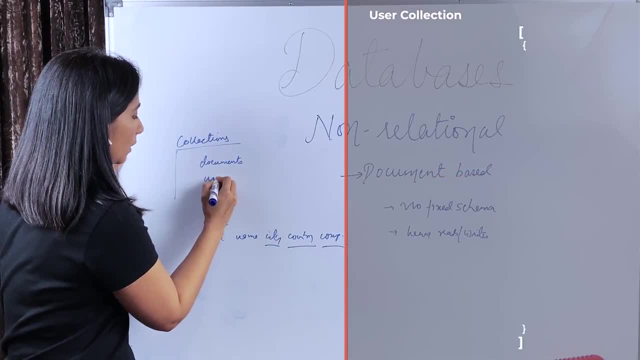 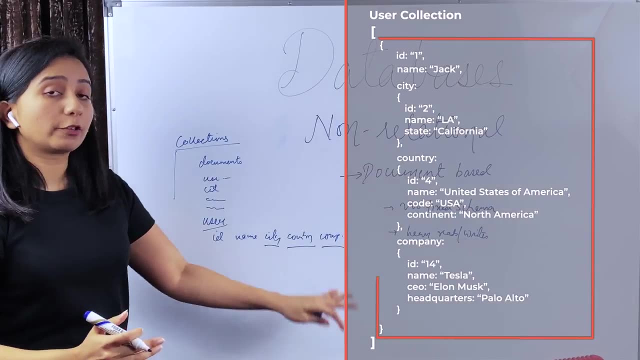 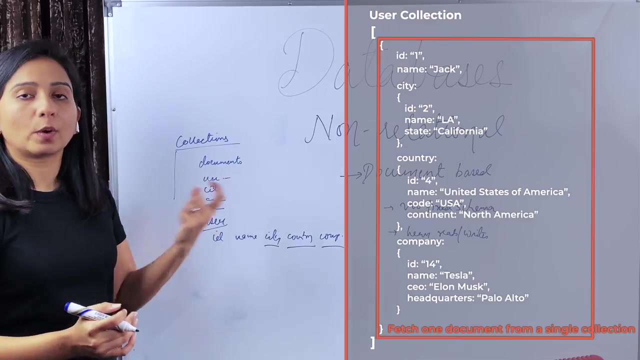 information in a document db where you have user and city and country and id. all that, all these details which are fetched from different tables. in case of relational db, if these are fetched, if these are stored in the document db itself, it just have to fetch one document. let's look at what are the downsides of document based. 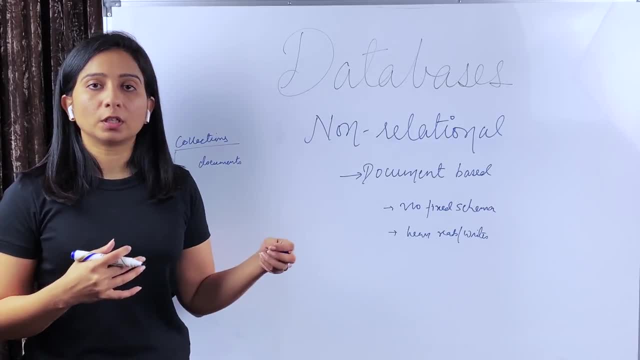 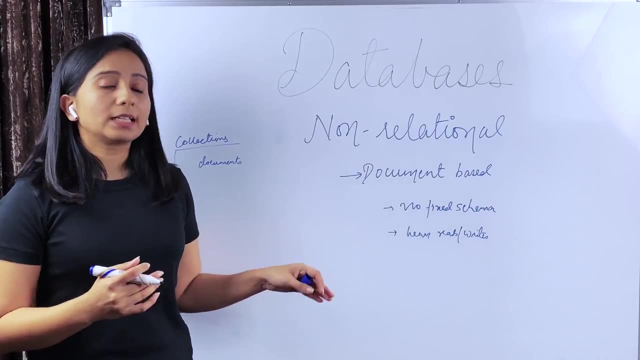 dbs. first, that you don't have schema, so you might have null values or empty values in your db if- and you have to- you might have to handle that in your application code. and second is these type of data that you provide as a transaction, so sometimes the updates could become complex and 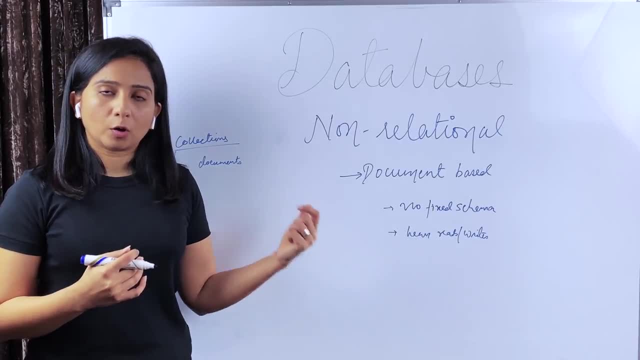 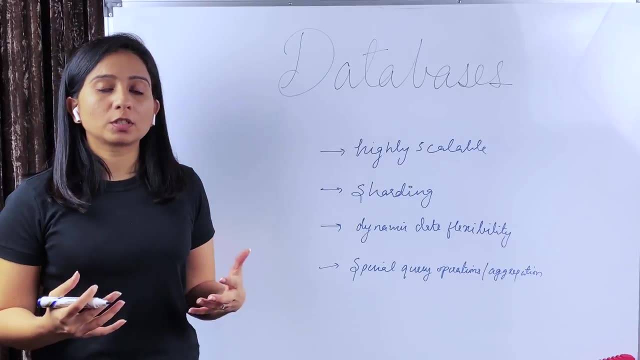 you cannot ensure if the transaction is completed or not completed, although you can handle that using application code, but that facility is not provided by the db itself. so to summarize some of the benefits or the reasons to choose a document: databases is they provide? they are highly scalable. 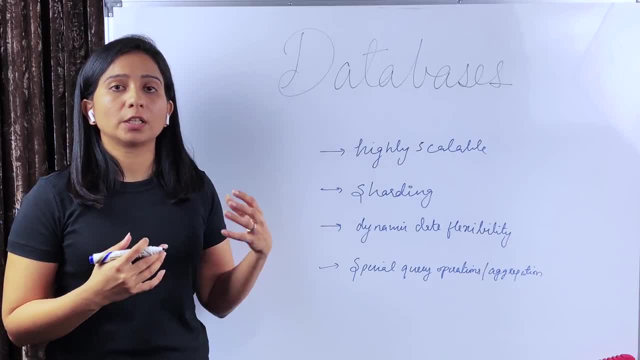 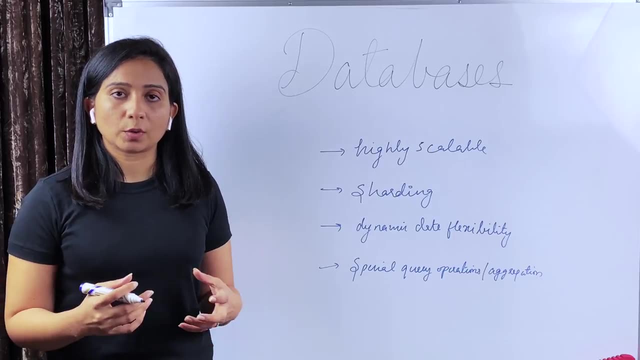 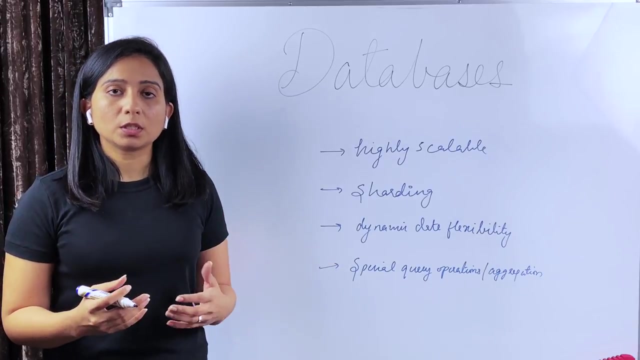 they provide sharding capabilities if you have dynamic data and you want that flexibility that you need a schema-less organization of your data. also provide special querying operations, aggregation queries that can help you to fetch data as per the requirement. when you have all these factors, no sql dbs or document dbs are one of the choices. 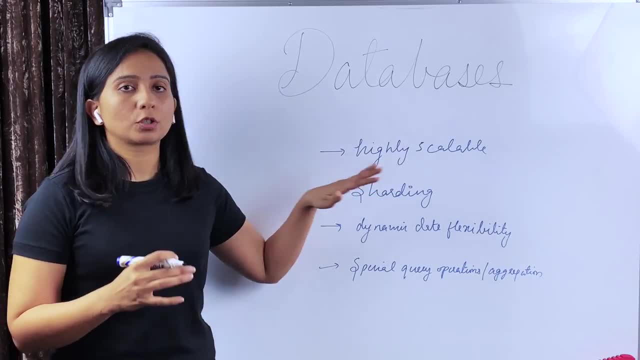 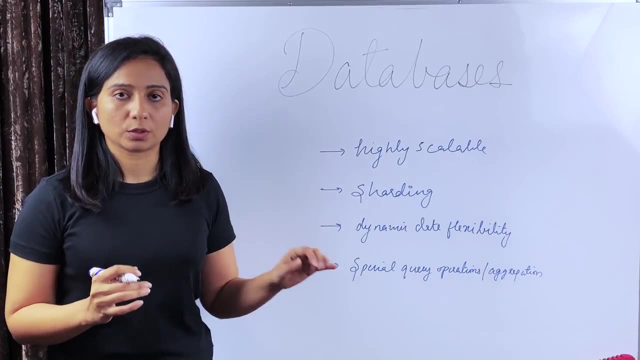 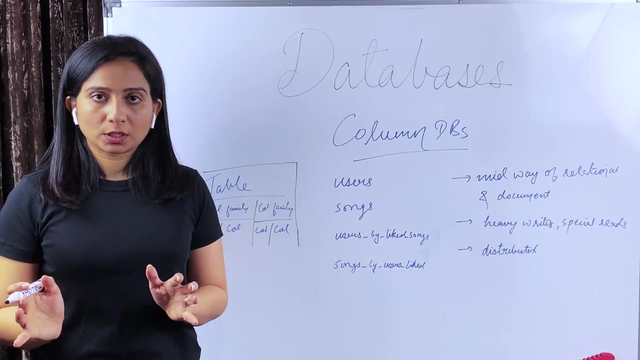 if you don't understand sharding or horizontal or vertical scaling. as i said, there are dedicated videos on this topic and we'll cover more about db sharding in those videos. now let's discuss what are column dbs or column wide stores. column dbs are sort of a midway of relational dbs and document. 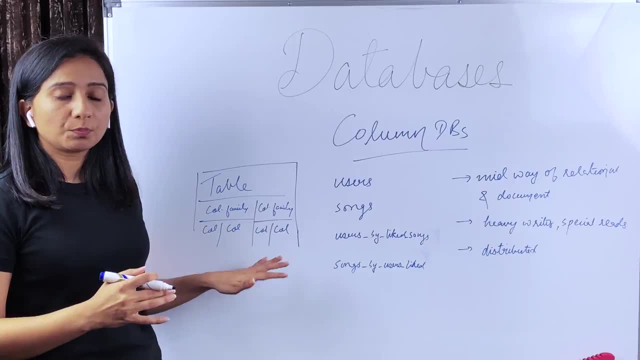 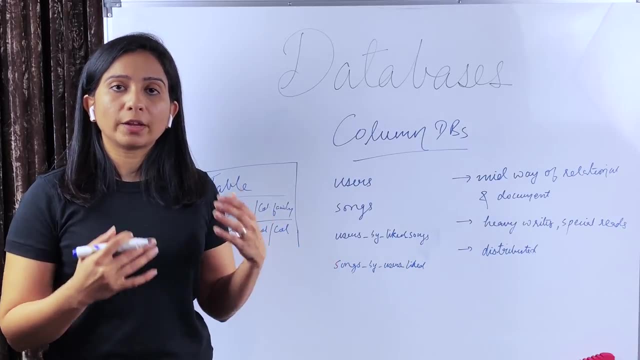 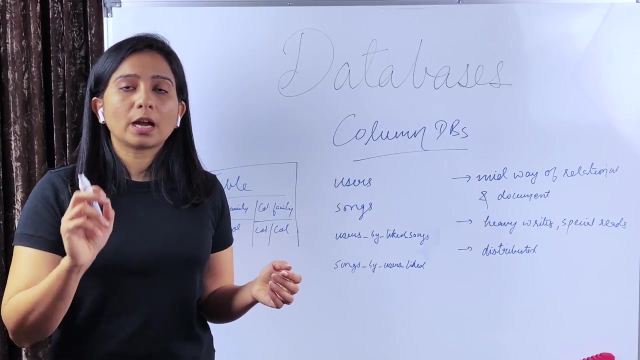 dbs are sort of a fixed schema with tables and columns, but these dbs do not support the asset transactions. also, such databases are used when you have a requirement of heavy reads. some examples are even data or streaming data. so if you use a music app, you are continuously either. 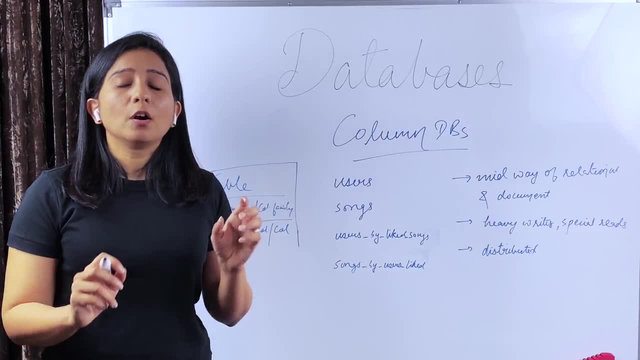 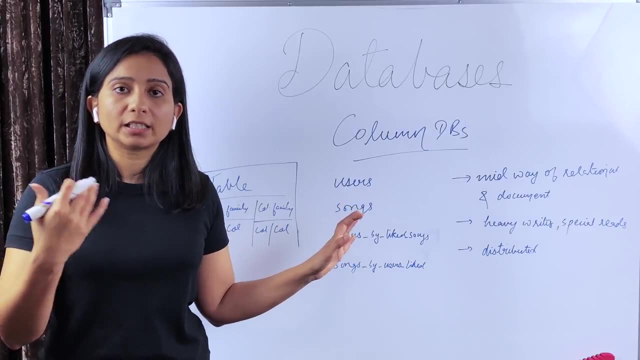 liking the mere song or skipping over the song favoriting your song. all those interactions that are doing have to be written and stored in dbs as even data, so that analytics could be run over them. so you can see that the data is stored in column dbs. some other examples could be storing health. 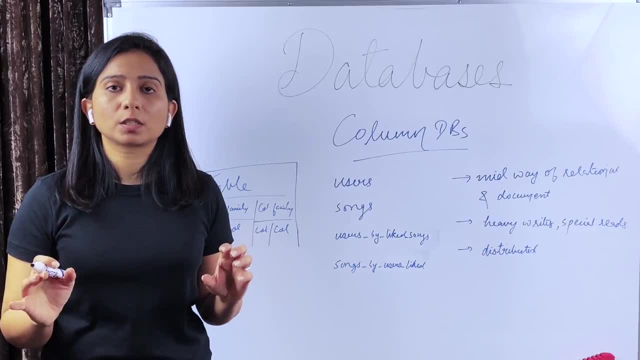 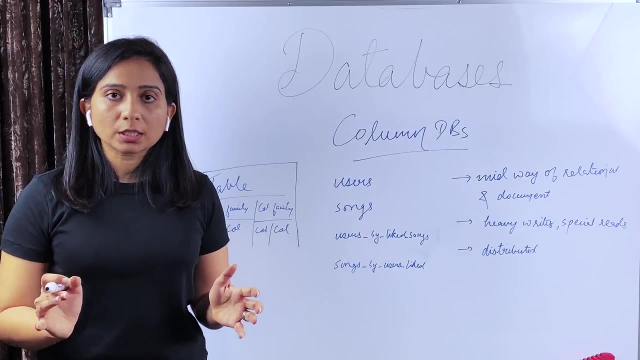 tracking data or storing data for iot devices where different sensors are deployed and sensors are sending data continuously within every 10 seconds or 30 seconds. in all such use cases, column dbs are used because they support a large number of heavy rights coming to the reads such dbs do. 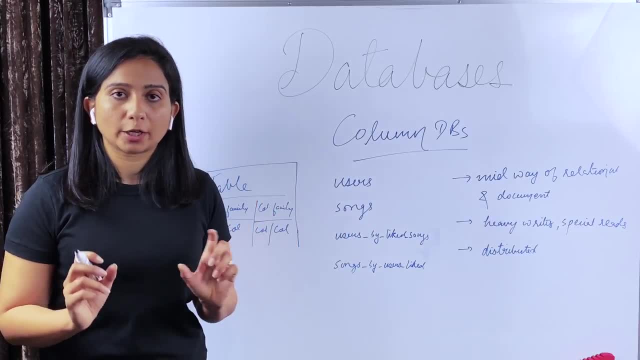 not support huge number of leads, but they do support a special kind of reads and the table structure is defined by the kind of data that is stored in column dbs. so in this case, column dbs is the kind of data that is stored in column dbs. so in this case, column dbs is the kind of data that is stored in column dbs. 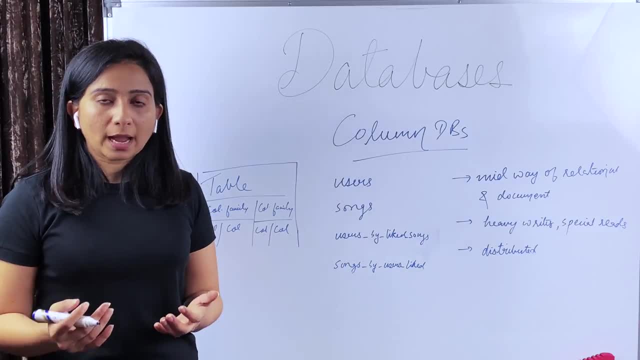 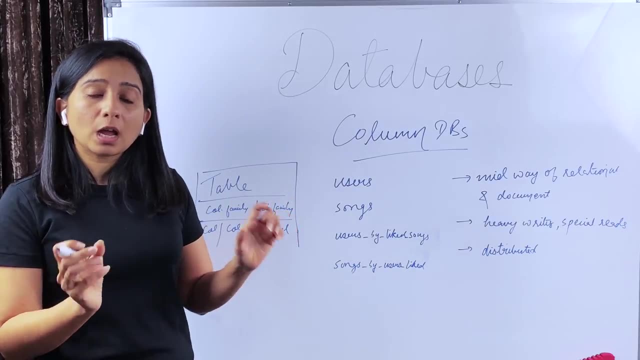 of queries you have to make, for example the music app. the queries will be: you have to fetch user detail, song detail. you have to fetch users that have liked the particular song and also you have to fetch the songs that are liked by a particular user. so some tables in column db could be then. 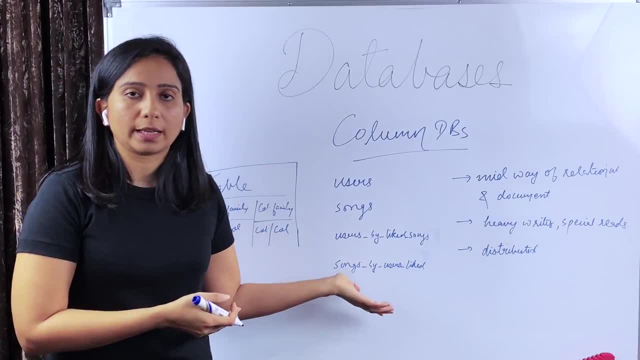 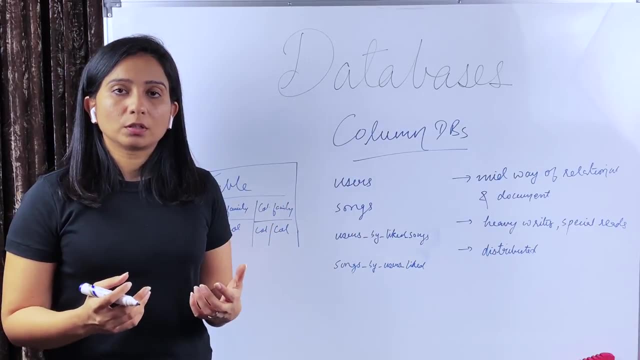 users, songs users by like songs and songs by users like. this design in column dbs is done with respect to what kind of reads are required. also, column dbs are a good supporter of distributed databases. if you don't know what are distributed databases, we will have a dedicated video on distributed dbs. 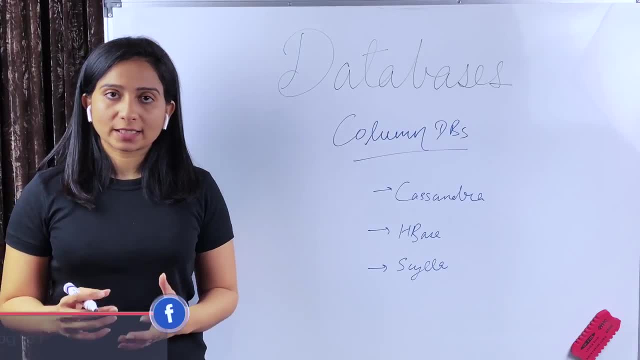 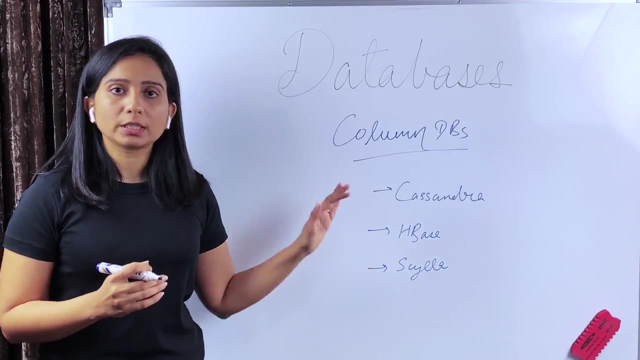 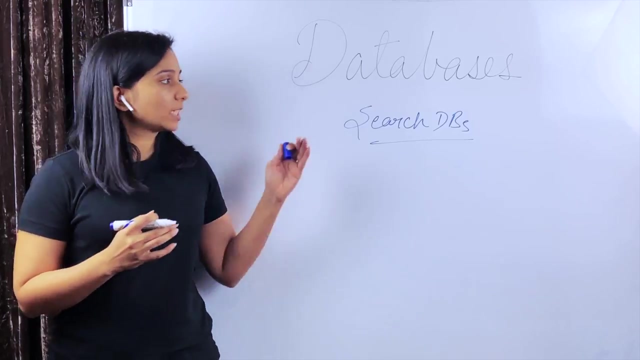 where we will dig into more of this in detail. some popular examples of column dbs are cassandra, hbase, sila, etc. in the description i have linked companies which use these databases and some more examples and use cases so that you understand how different companies are using these dbs. now let's talk about search databases. whenever you interact with any 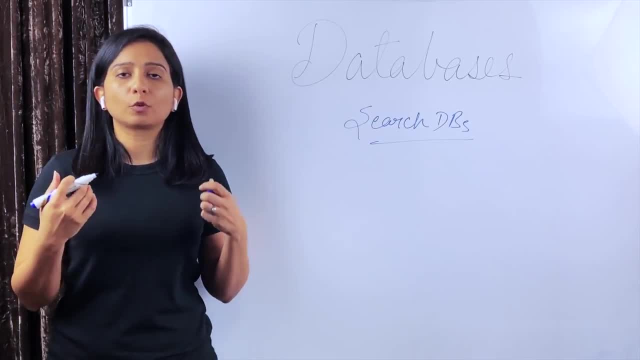 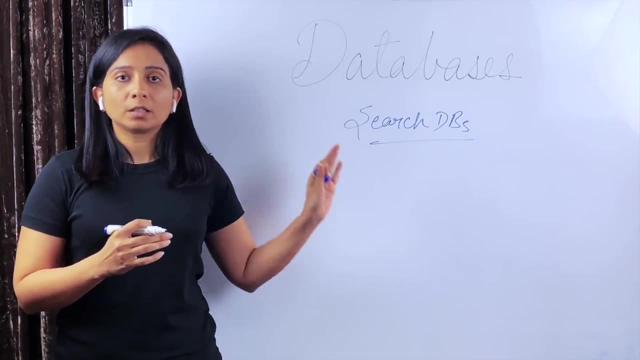 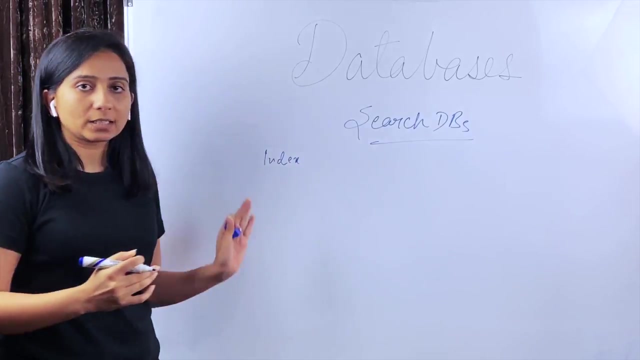 application where you search for something like for booking a flight, or for booking a movie, or if you're purchasing an item on amazon. all those full text search queries are supported by data stored in search databases. for example, if you're reading a book, you usually have an index. 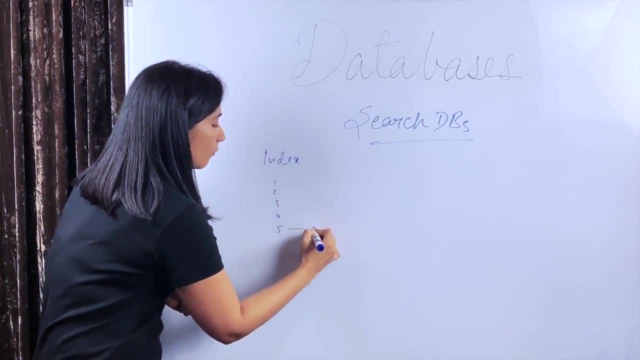 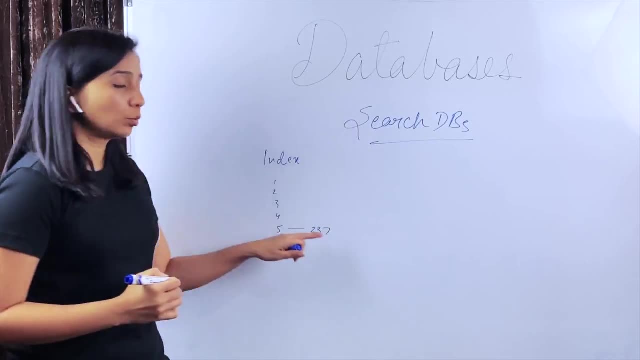 at the starting of the book you can find out where, uh, every chapter can be accessed. so suppose if you want to go to chapter 5, it will say: okay, go to page 237. so that's how you can easily access this page. similarly, the data against those queries. 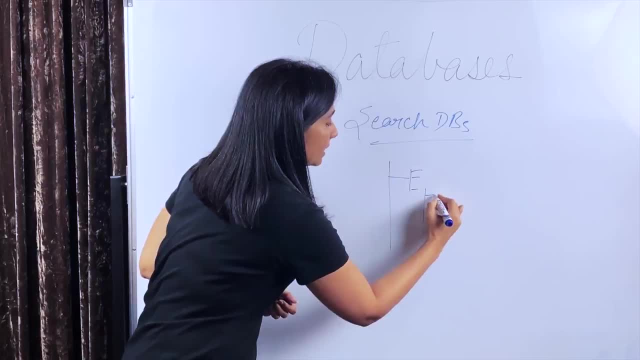 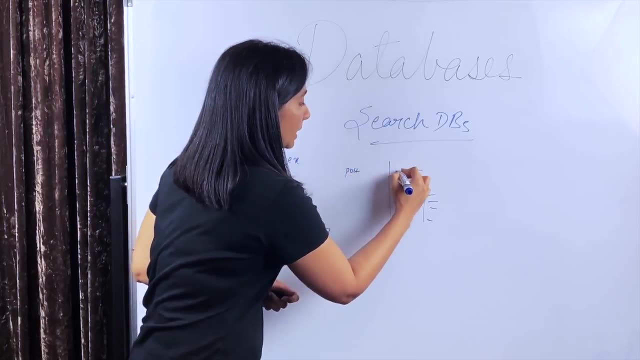 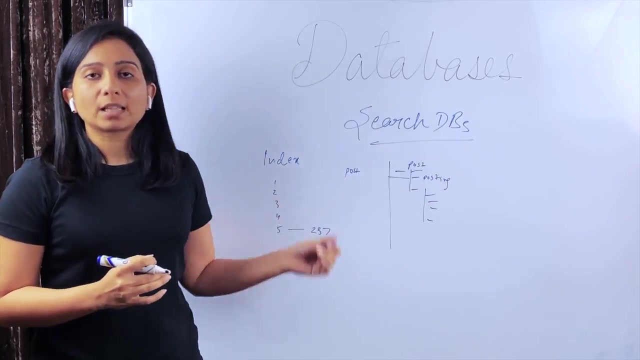 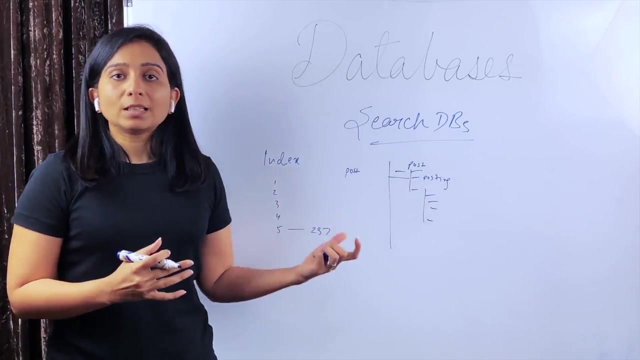 are is stored in advanced indexes inside search databases. so when you search for a particular item, say, post it, there will be data saved in these indexes to support those search queries. some example of search databases are elastic, so solar, etc. the important thing to note here is the data that is stored in search databases. that is not the primary data store. so if 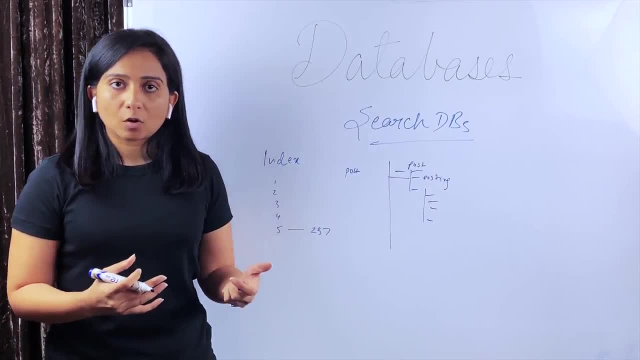 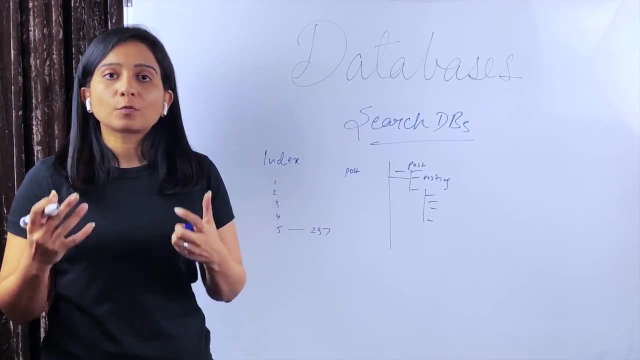 you are working with an e-commerce application, the product catalog. all the products and items will be stored in a primary database, maybe a relational or a non-relational db, and the results of search queries or the data on which frequent queries are executed, that will be stored on search. 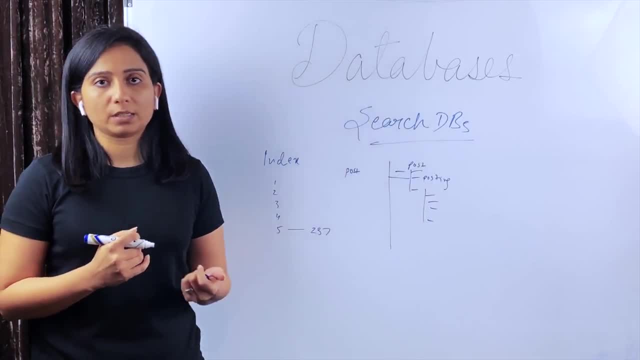 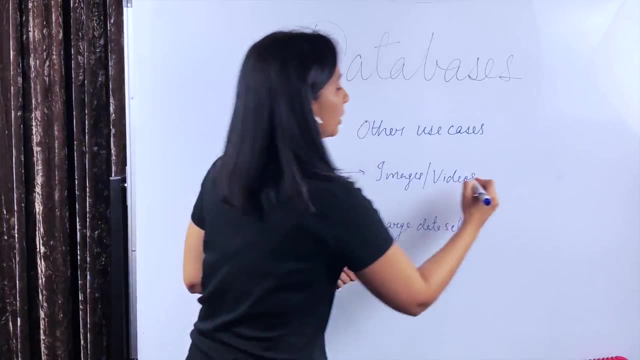 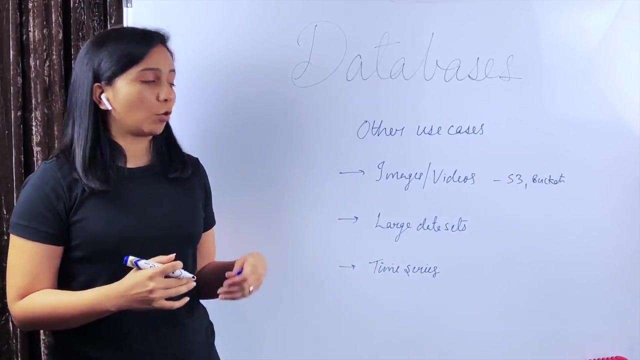 db and it will be refreshed as per the frequency of the queries. some other use cases for data are images and videos. such a kind of data is stored usually on cloud, in amazon s3 or buckets in case one is using gcp. then there are large data sets, or time series data, where a lot of data has to be. 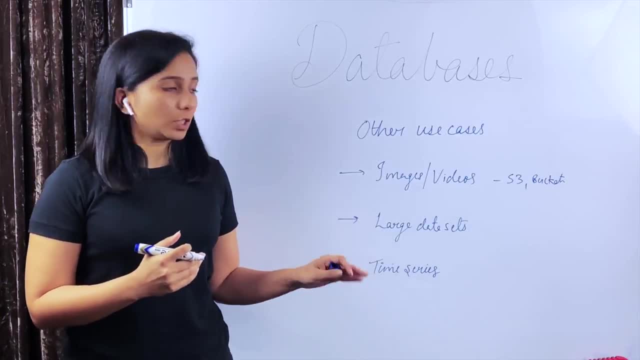 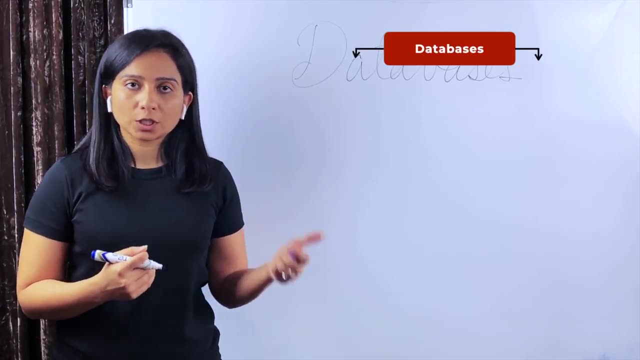 stored and analytics is run over that. there are different kind of databases which cater to such needs. all the details are included in the description. so the types of dbs and different use cases that we have just discussed- these are the most popular ones. there are many more types.